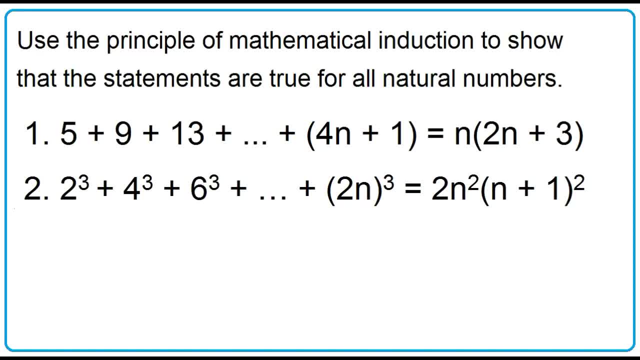 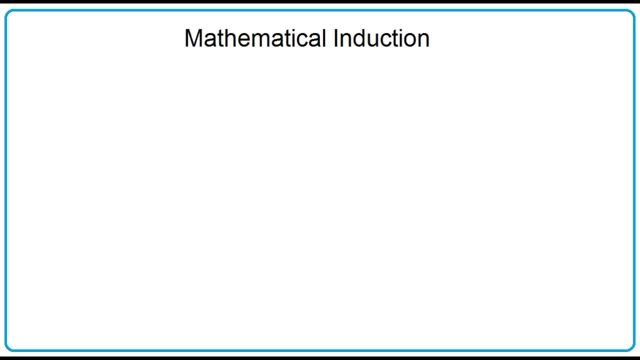 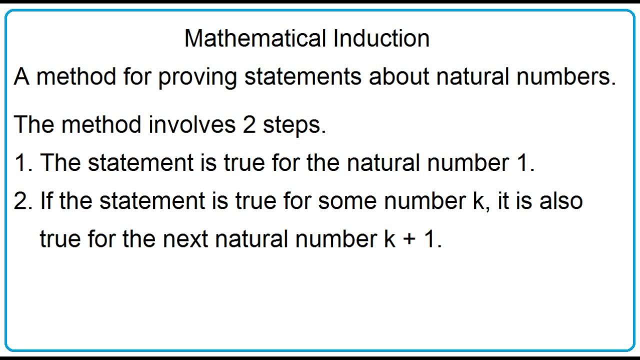 Use the principle of mathematical induction to show that the statements are true for all natural numbers. What is mathematical induction? It is a method for proving statements about natural numbers. The method involves two steps. One: the statement is true for the natural number 1.. Two: if the statement is true for some number k, it is also true for the next. 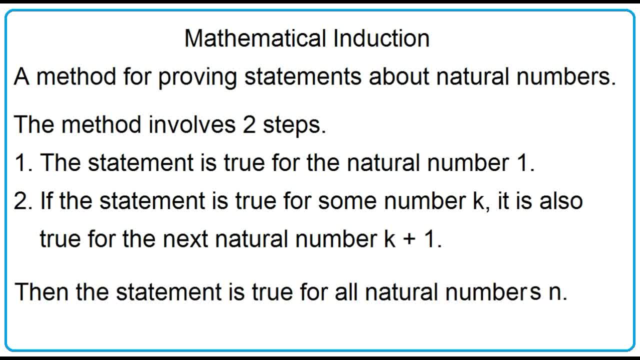 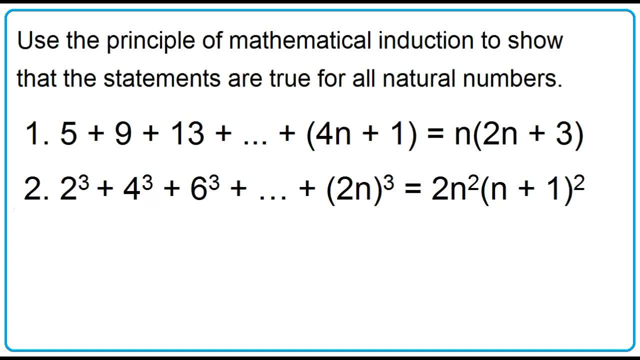 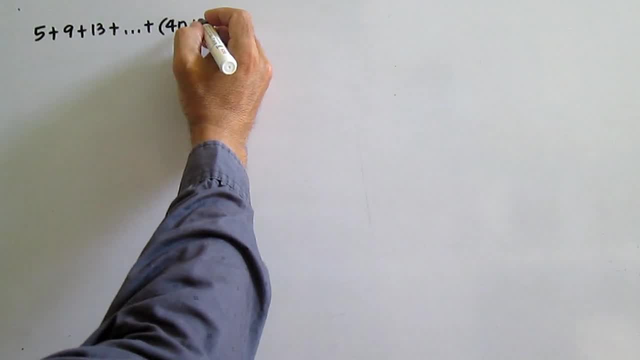 natural number k plus 1.. Then the statement is true for all natural numbers n. Let's use the principle of mathematical induction to show that the statements are true for all natural numbers: Number 1,, 5 plus 9 plus 13 plus dot, dot, dot, plus the quantity 4n plus 1. 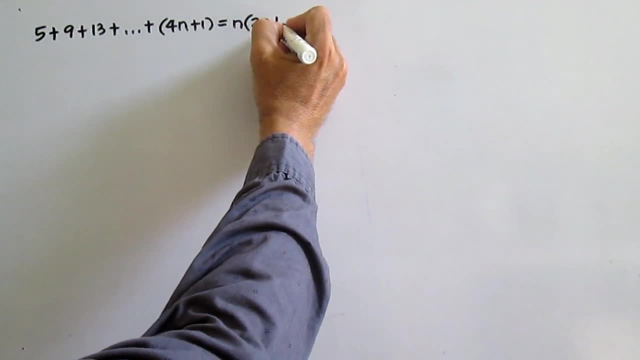 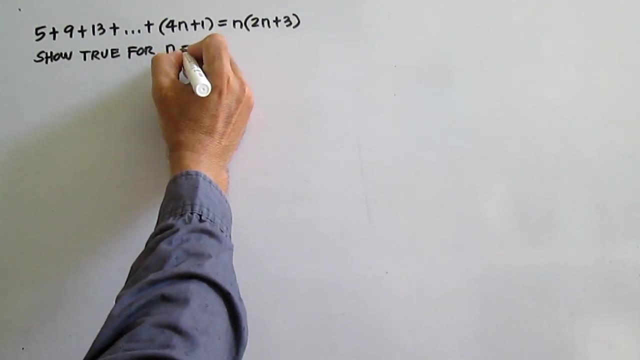 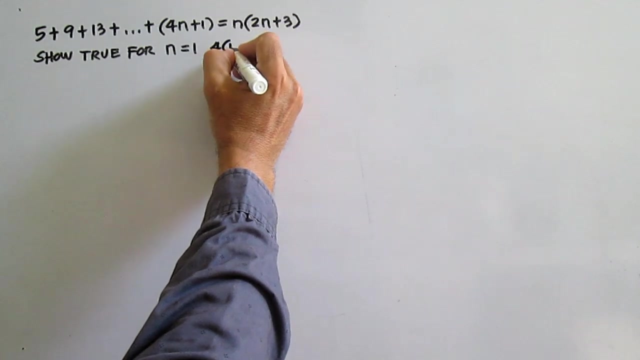 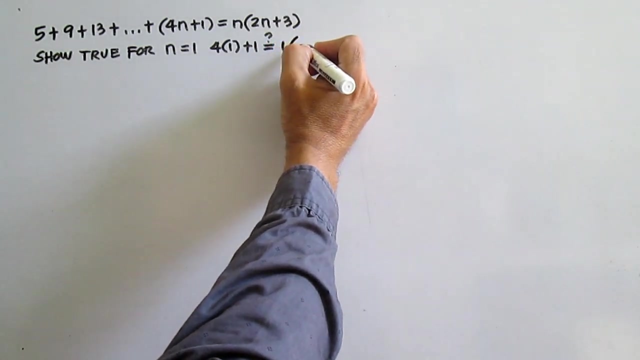 is equal to n times the quantity 2n plus 3.. Show that the statement is true: for n equals 1.. Substitute 1 for n for the expression 4n plus 1.. Is 4 times 1 plus 1 equal to 1 times the quantity 2 times 1 plus 3?. 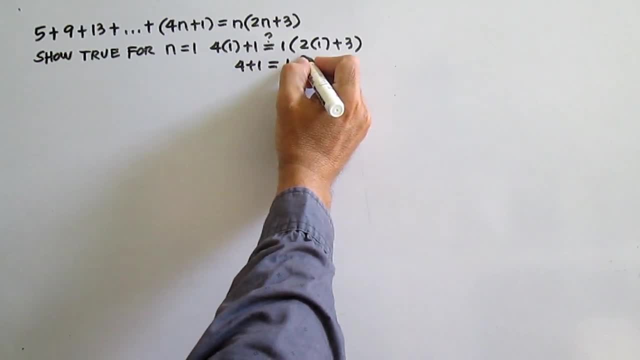 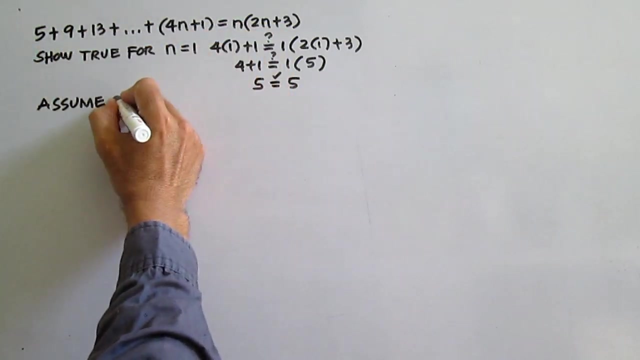 4 plus 1 is equal to 1 times the quantity 2 times 1 plus 3.. The quantity 2 plus 3 is 5.. 5 equals 5. True. Assume that the statement is true for any natural number k. 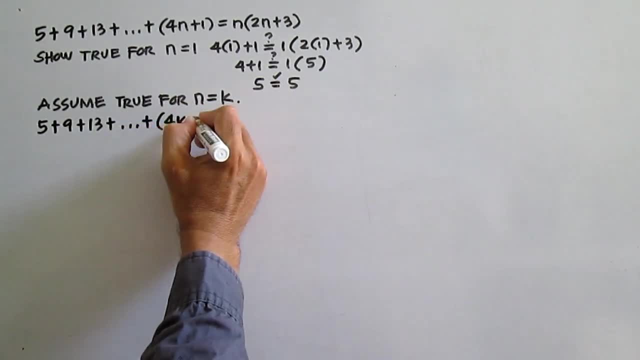 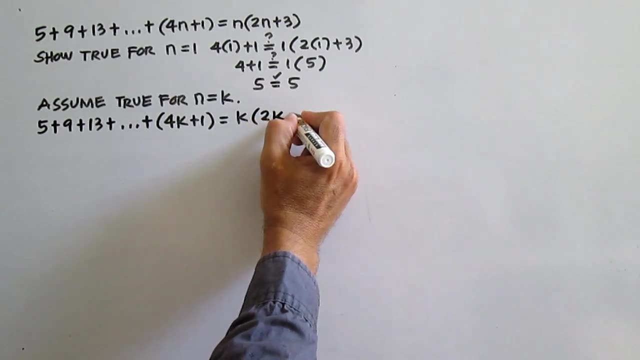 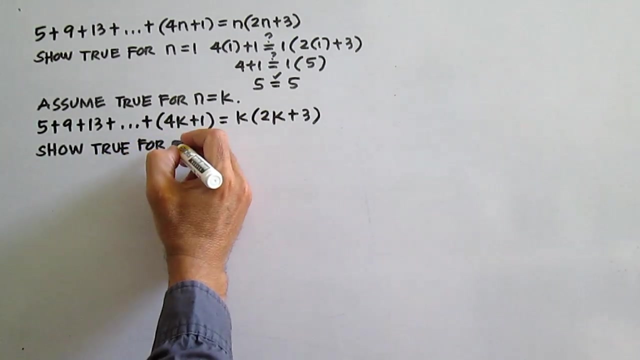 Substitute k for n, The quantity 4k plus 1. Is equal to k times the quantity 2k plus 3.. Show that the statement is true for the next natural number. Show true for: n equals k plus 1.. 5 plus 9 plus 13 plus dot, dot, dot plus 4k plus 1.. 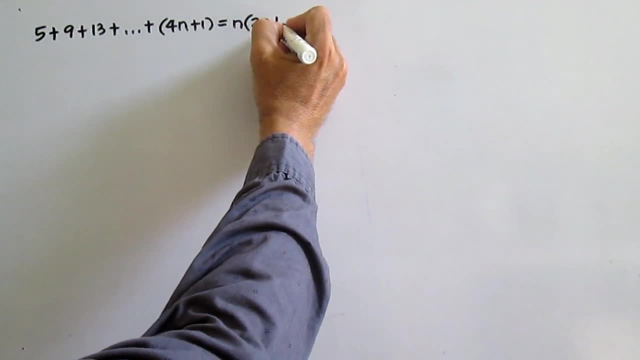 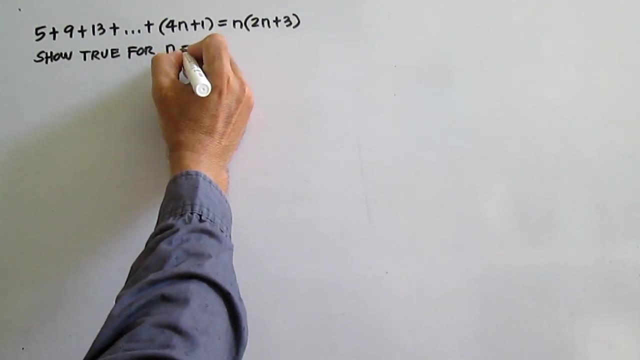 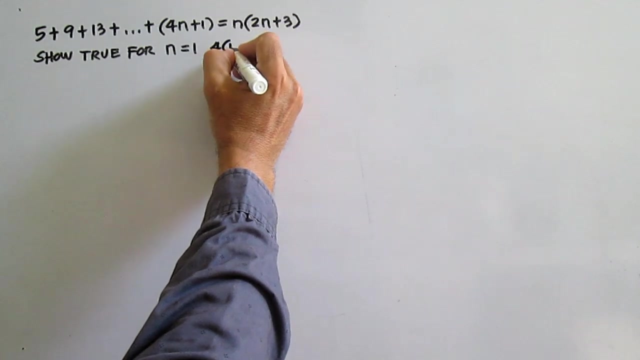 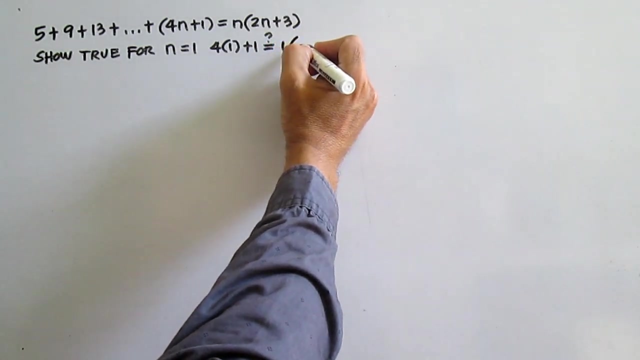 is equal to n times the quantity 2n plus 3.. Show that the statement is true: for n equals 1.. Substitute 1 for n for the expression 4n plus 1.. Is 4 times 1 plus 1 equal to 1 times the quantity 2 times 1 plus 3?. 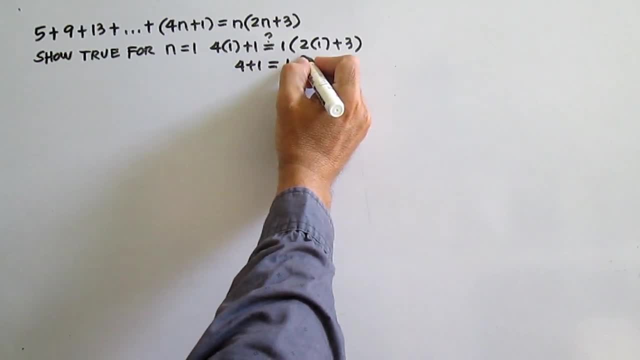 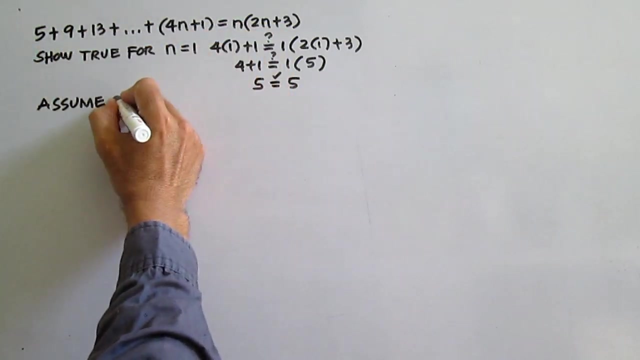 4 plus 1 is equal to 1 times the quantity 2 times 1 plus 3.. The quantity 2 plus 3 is 5.. 5 equals 5. True. Assume that the statement is true for any natural number k. 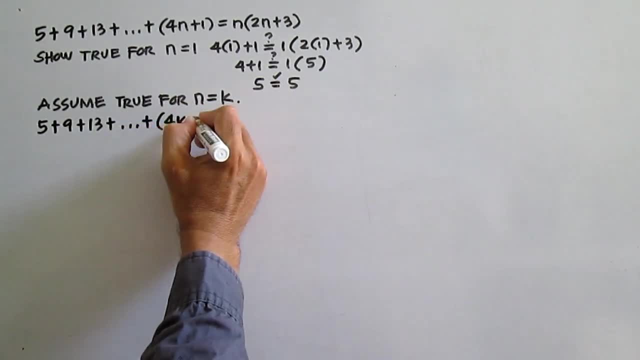 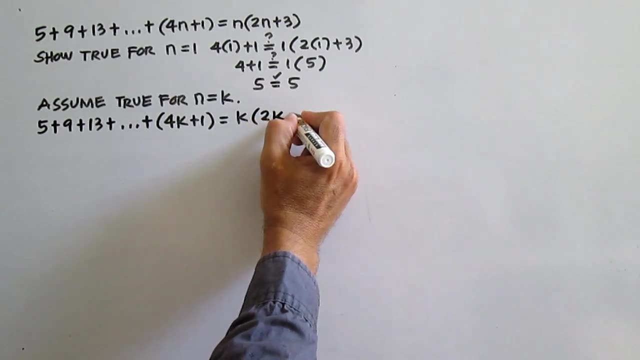 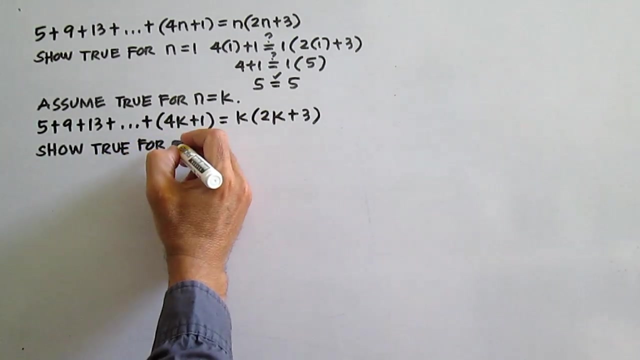 Substitute k for n, The quantity 4k plus 1. Is equal to k times the quantity 2k plus 3.. Show that the statement is true for the next natural number. Show true for: n equals k plus 1.. 5 plus 9 plus 13 plus dot, dot, dot plus 4k plus 1.. 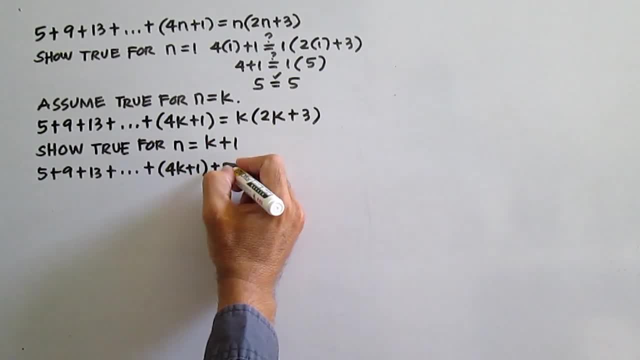 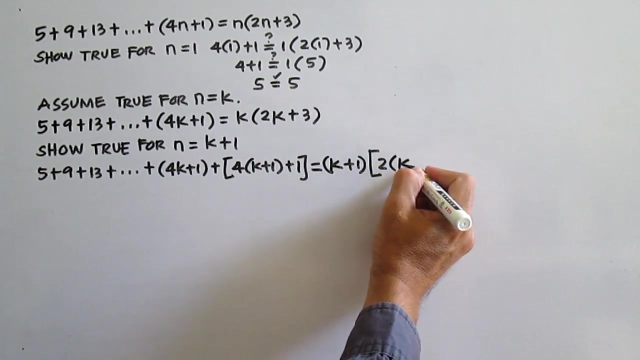 Plus. the next term is the quantity 4.. Substitute k plus 1 for n Is equal to k plus 1 times the quantity 2 times k plus 1 plus 3. Note that this expression is equal to the left hand side of our assumption. 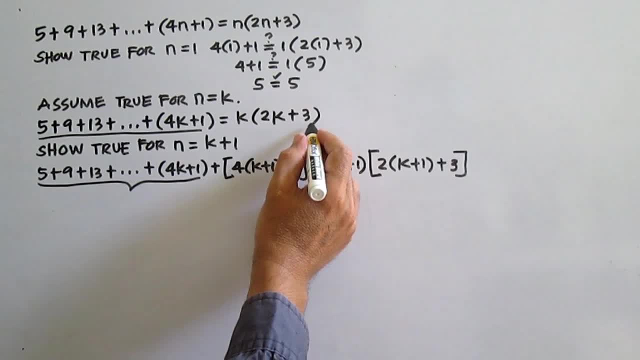 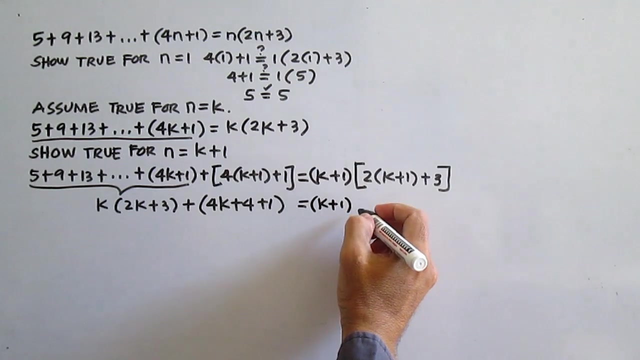 which is equal to k times the quantity 2k plus 3. Let's substitute k times the quantity 2k plus 3 plus 4k plus 4 plus 1 is equal to k plus 1 times 2k plus 2 plus 3. 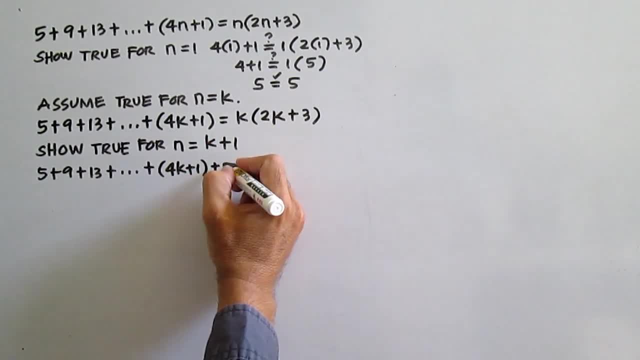 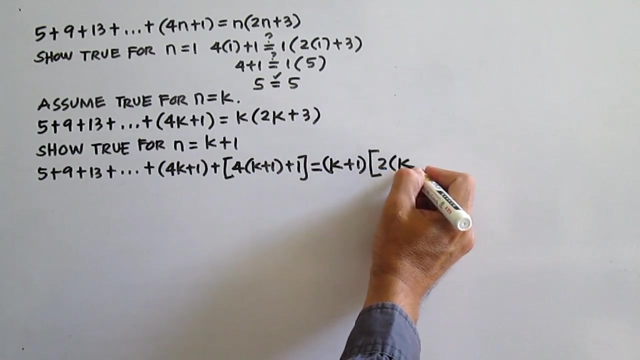 Plus. the next term is a quantity 4. substitute k plus 1 for n. Substitute k for n Is equal to times the quantity 2 times k plus 1 plus 3.. Note that this expression is equal to the left-hand side of our assumption. 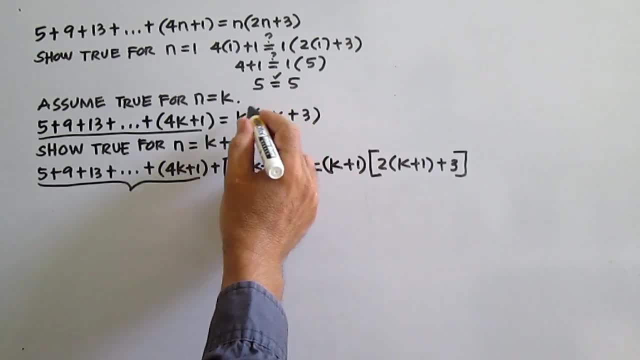 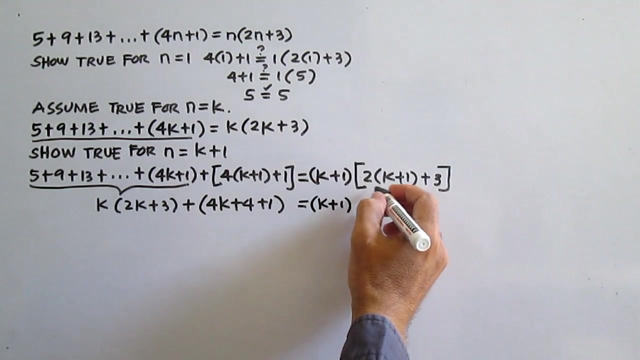 which is equal to k times the quantity 2k plus 3.. Let's substitute k times the quantity 2k plus 3 plus 4k plus 4 plus 1 is equal to k plus 1 times 2k plus 2 plus 3.. 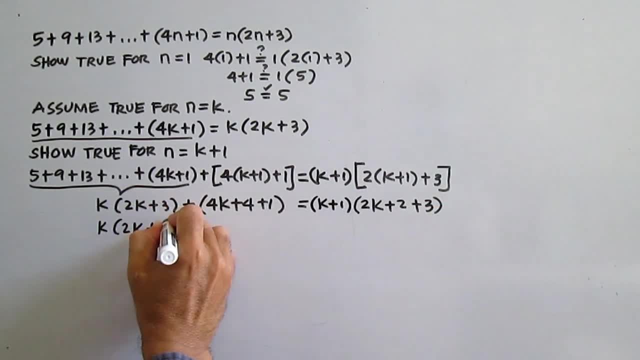 Let us show that the left-hand side of the equation is equal to the right-hand side of the equation: is k times the quantity 2k plus 3 plus the quantity 4k plus 5, is equal to the quantity k plus 1 times the quantity 2k plus 5.. 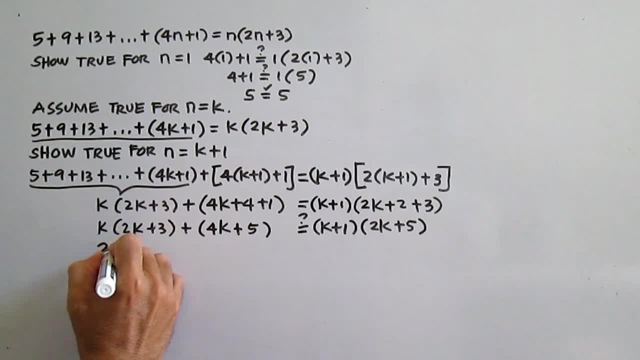 k times the quantity 2k plus 3 is equal to 2k squared plus 3k plus 4k plus 5 is equal to k plus 1 times the quantity 2k plus 5.. Combine similar terms: 2k squared plus 7k plus. 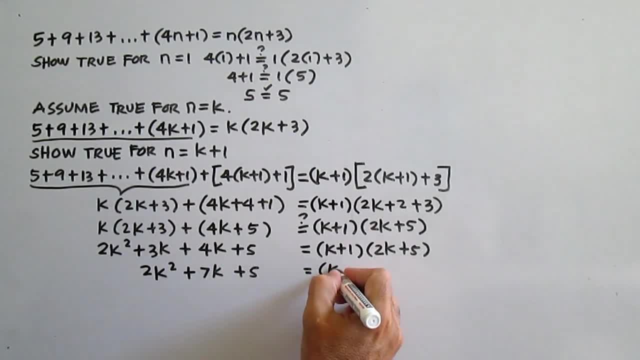 k plus 5 is equal to the quantity k plus 1 times the quantity 2k plus 5.. The factors of 2k squared plus 7k plus 5 is equal to the quantity k plus 1 and the quantity 2k plus 5.. 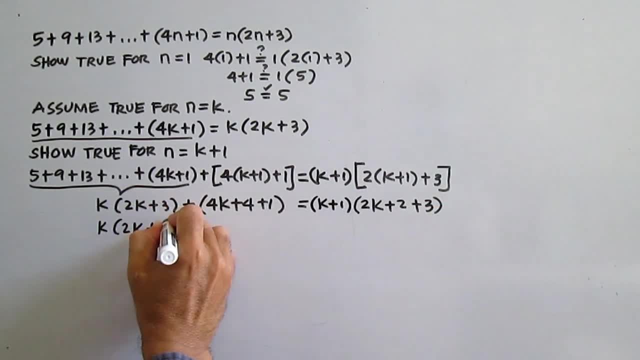 Let us show that the left hand side of the equation is equal to the right hand side of the equation: is k times the quantity 2k plus 3 plus the quantity 4k plus 5. is equal to the quantity k plus 1 times the quantity 2k plus 5. 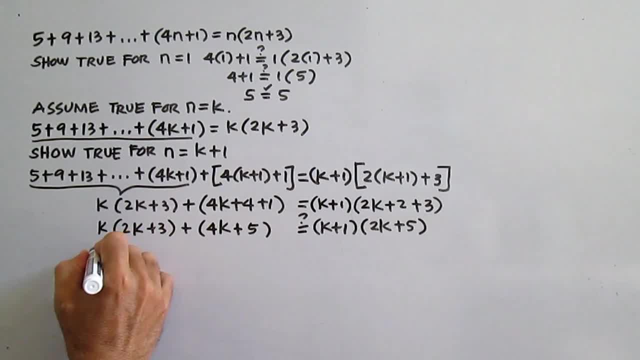 k times the quantity 2k plus 3 is 2k squared plus 3k plus 4k plus 5 is equal to k plus 1 times the quantity 2k plus 5. Combine similar terms: 2k squared plus 7k. 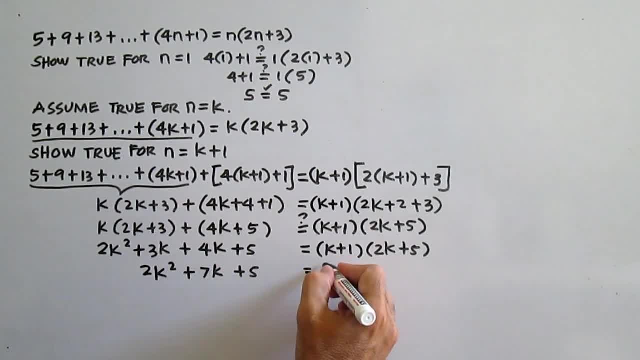 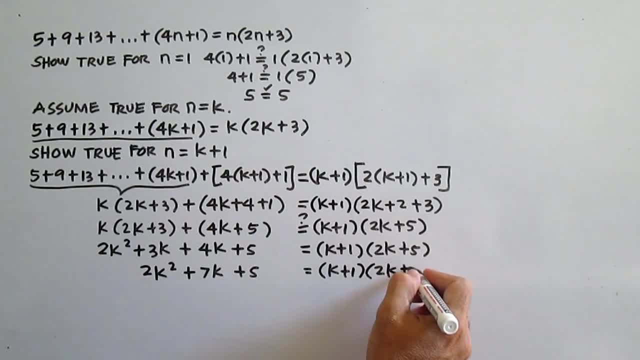 times the quantity 2k plus 5. the factors of 2k squared plus 7k plus 5 is equal to the quantity k plus 1 and the quantity 2k plus 5. this is equal to the quantity k plus 1. 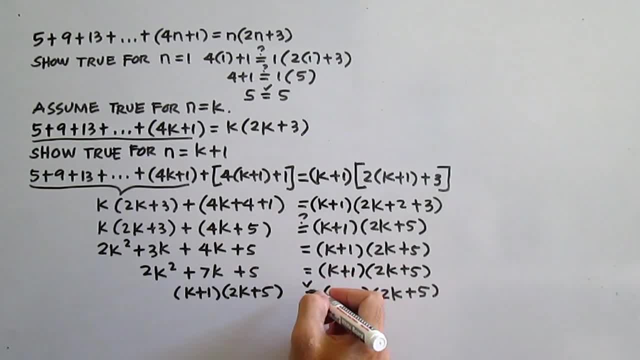 times the quantity 2k plus 5. 2k plus 5. true therefore, the statement: 5 plus 9 plus 13 plus dot, dot, dot plus the quantity 4n plus 1 is equal to n times the quantity 2n plus 3. is true for all natural numbers n. 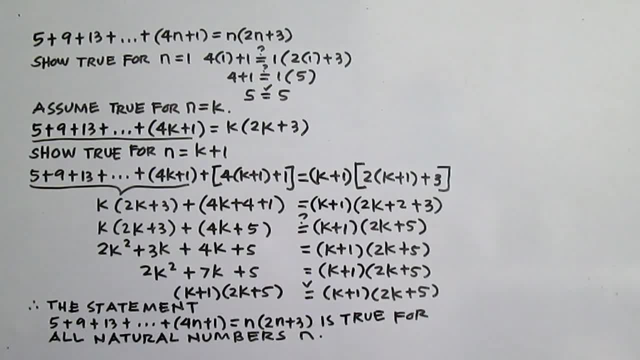 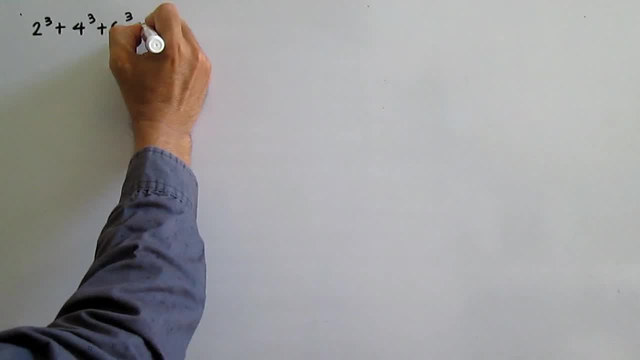 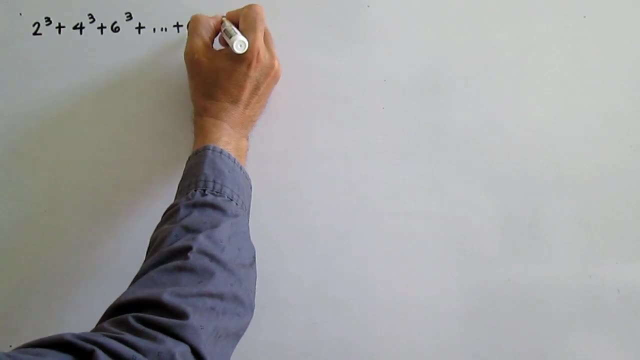 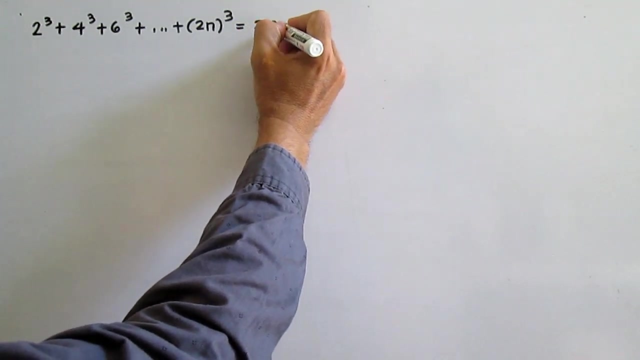 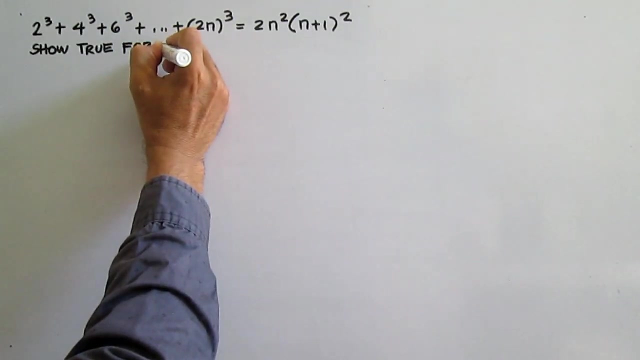 use the principle of mathematical induction to show that the statement 2 cubed plus 4 cube plus 6 cube plus dot dot dot plus the cube of 2n equals 2n squared times the square of the quantity n plus 1. show that the statement is true for n equals 1. 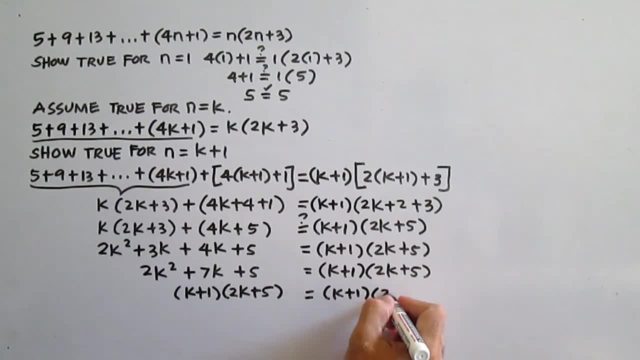 This is equal to the quantity k plus 1 times the quantity k plus 1 times the quantity 2k plus 5.. True, Therefore, the statement 5 plus 9 plus 13, plus dot, dot, dot, plus the quantity 4n plus 1. 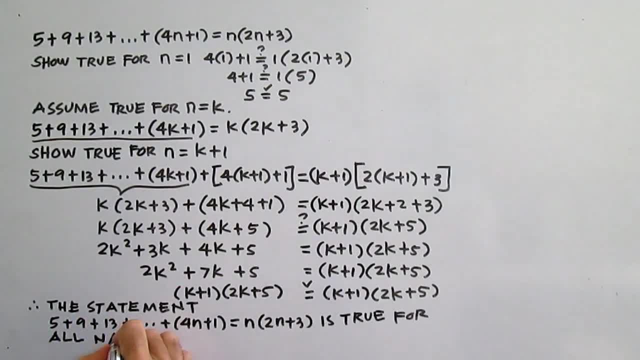 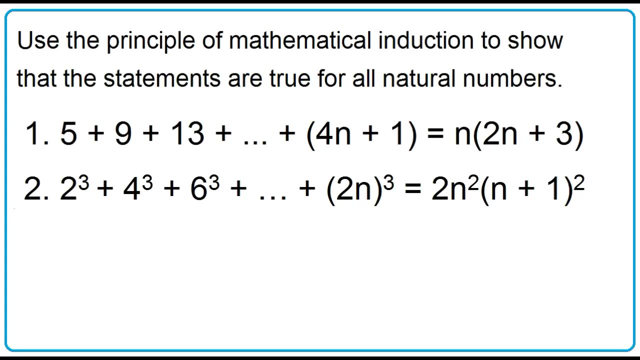 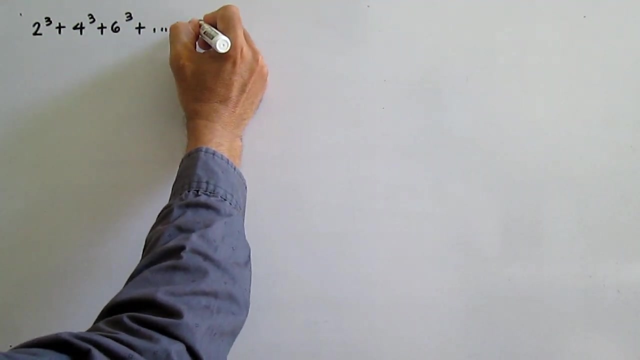 is equal to n times the quantity 2n plus 3 is true for all natural numbers n. Use the principle of mathematical induction to show that the statement 2 cubed plus 4 cube plus 6 cube plus dot, dot, dot plus the. 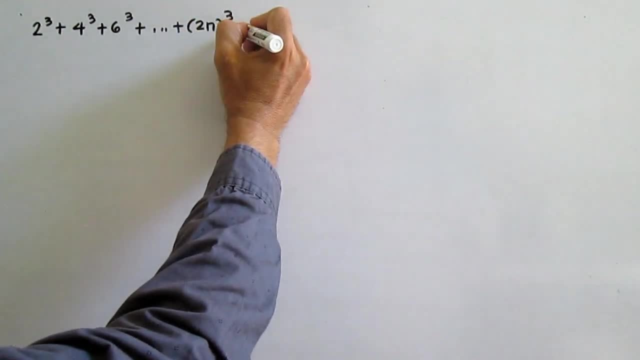 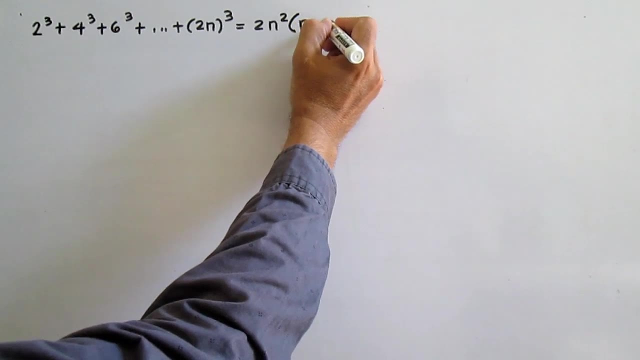 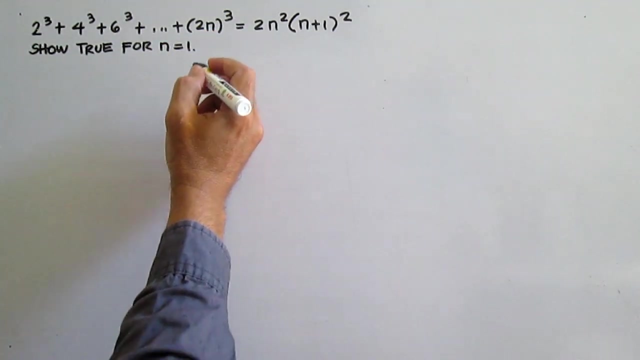 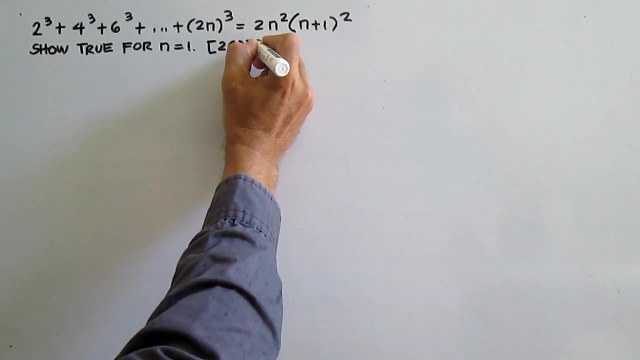 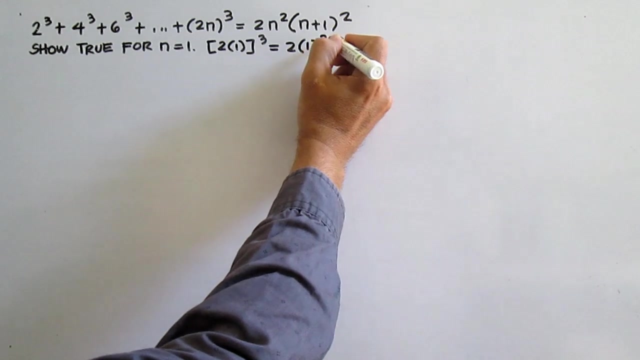 cube of 2n equals 2n squared times the square of the quantity n plus 1. show that the statement is true. for n equals 1. substitute 1 for n. a cube of 2 times 1 is equal to 2 times the square of 1 times. 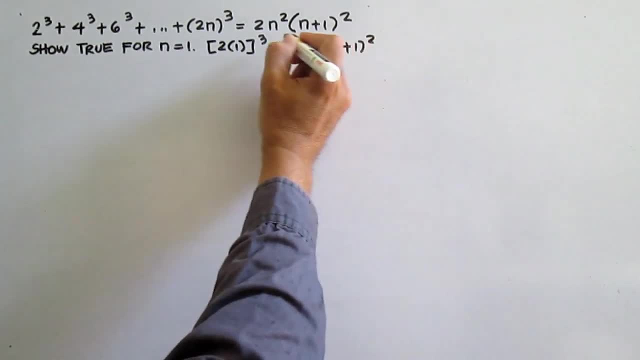 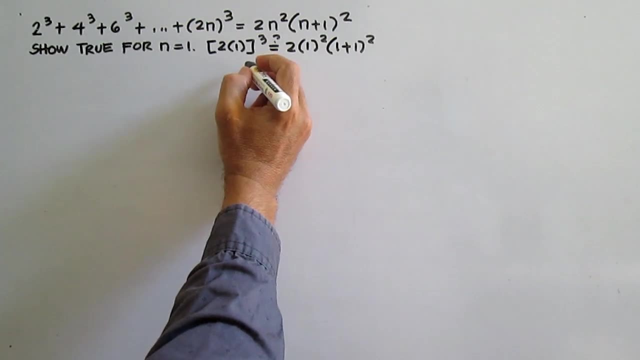 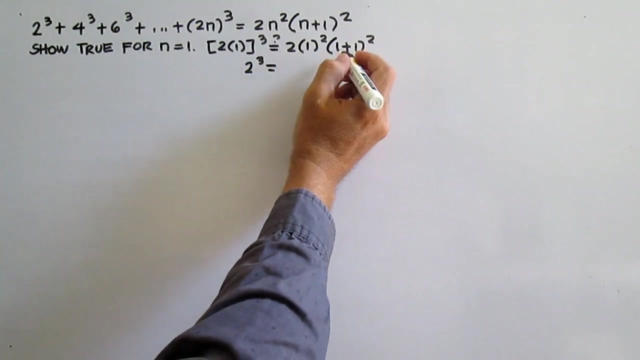 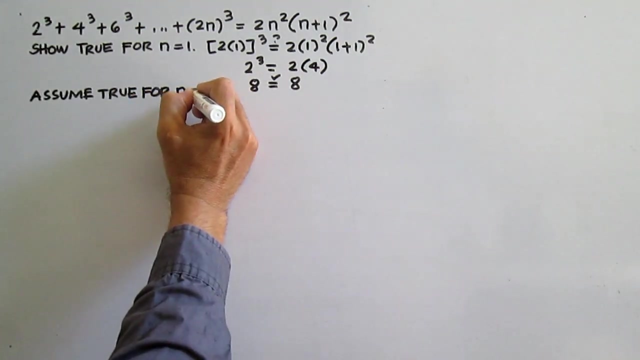 the square of 1 plus 1, is the left-hand side equal to the right-hand side of the equation. 2 cubed is equal to 2 times 4. 8 is equal to 8. true. assume that the statement is true for any natural number k. 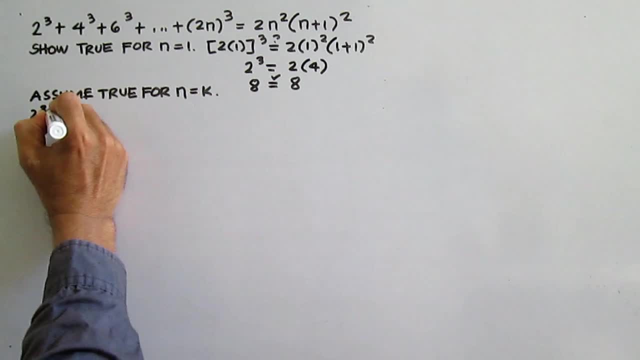 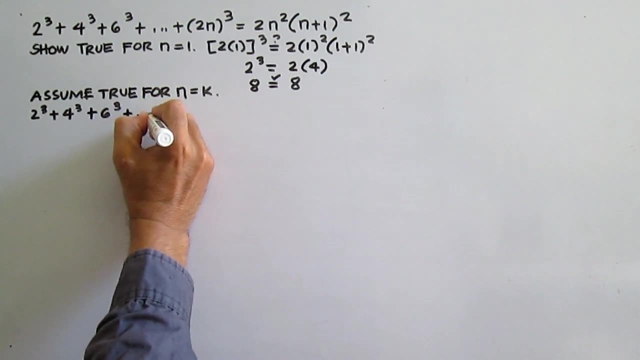 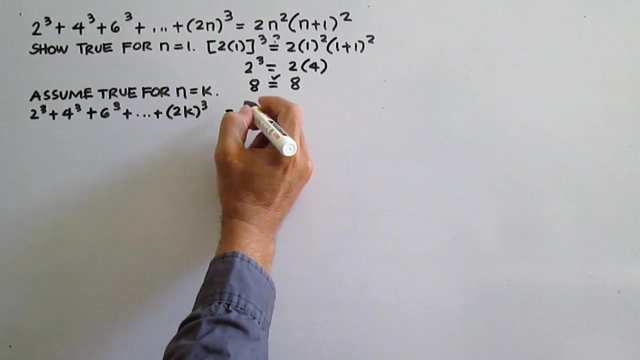 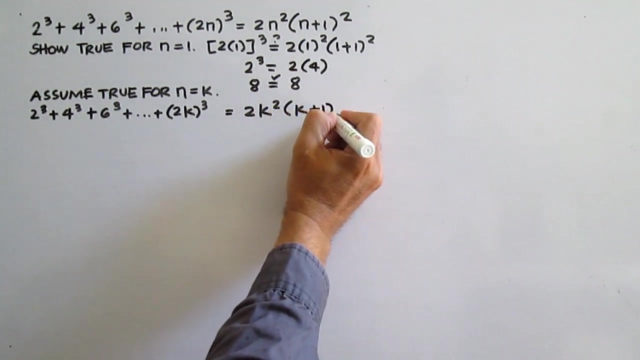 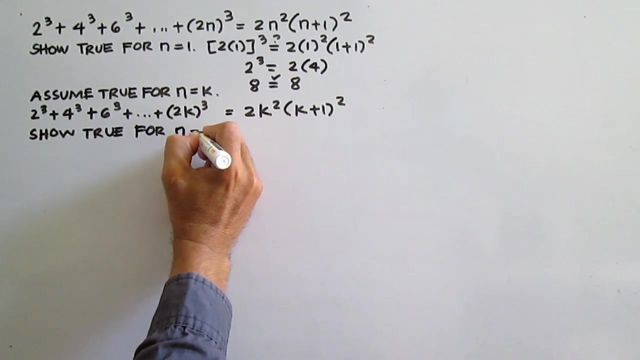 substitute k for n. 2 cubed plus 4 cube plus 6 cubed plus dot dot dot plus the quantity 2 K cubed is equal to 2 K squared times the square of K plus 1. show that the statement is true for the next natural number. show true for n. 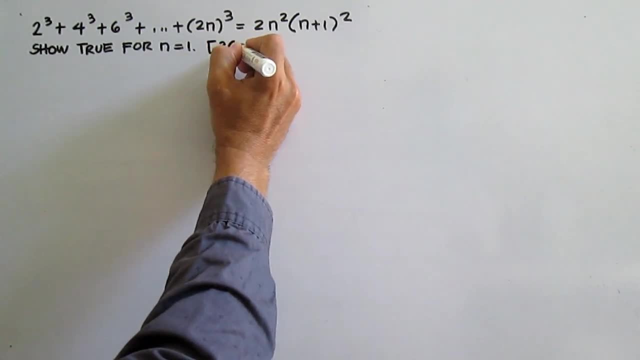 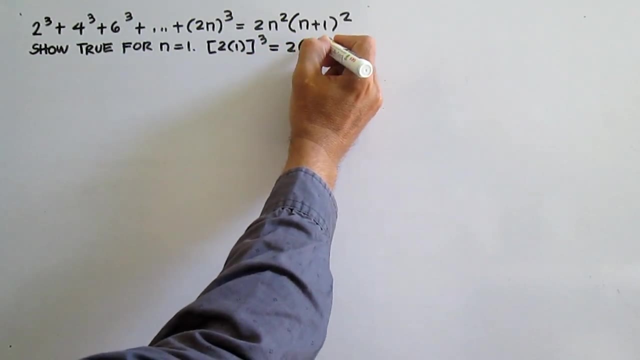 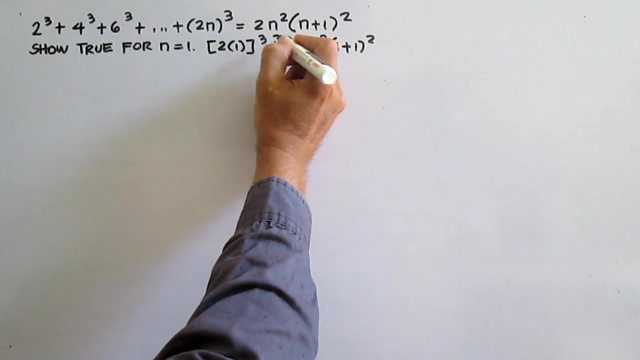 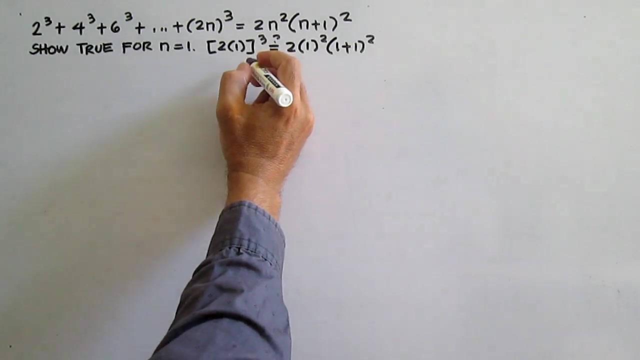 substitute 1 for n. a cube of 2 times 1 is equal to 2 times the square of 1 times the square of 1 plus 1 is the left-hand side equal to the right-hand side of the equation. 2 cubed is equal to. 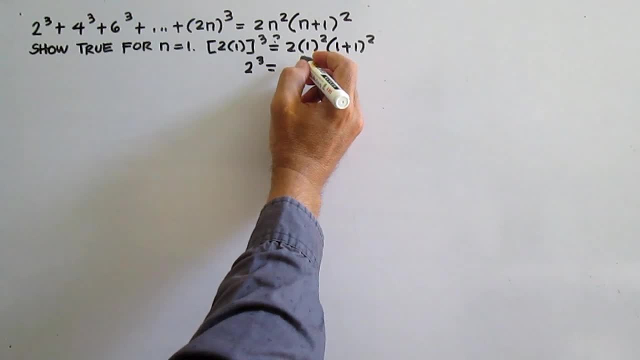 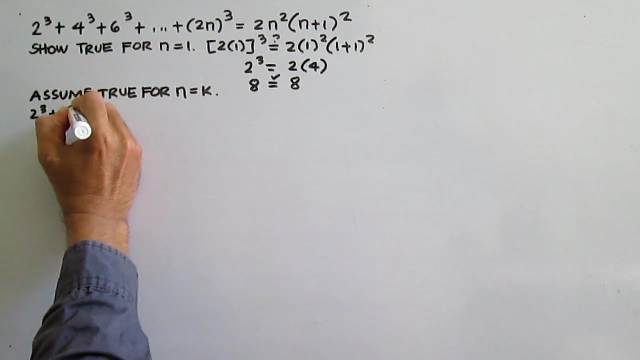 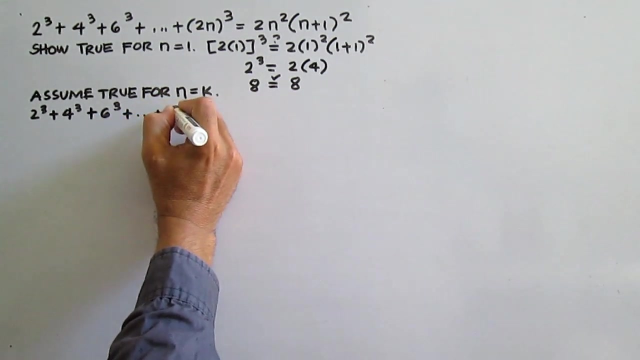 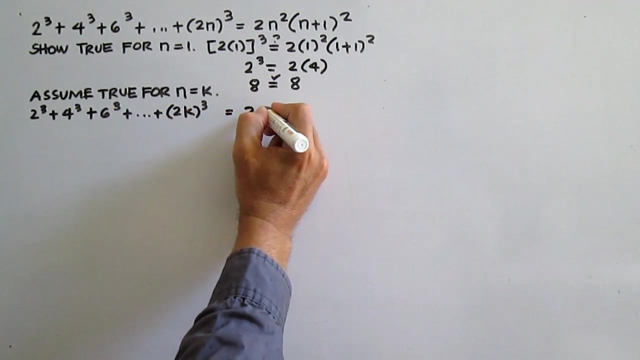 2 times 4, 8 is equal to 8. true. assume that the statement is true for any natural number. substitute K for n. 2 cube plus 4 cube plus 6 cubed plus dot, dot, dot plus the quantity. 2 K cubed is equal to 2 K squared times the square of K plus 1. 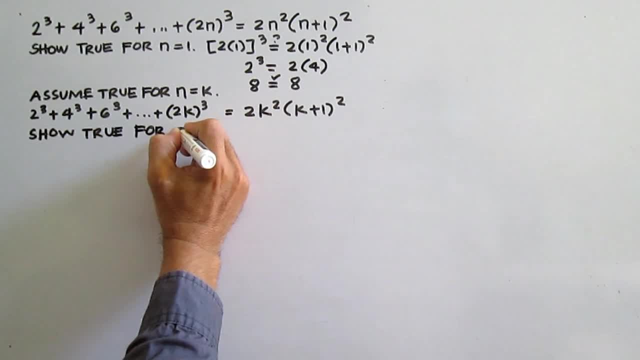 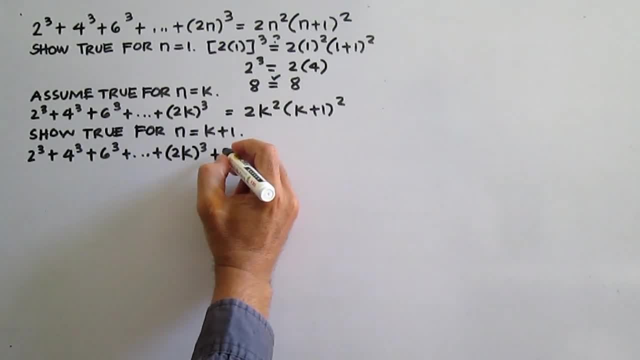 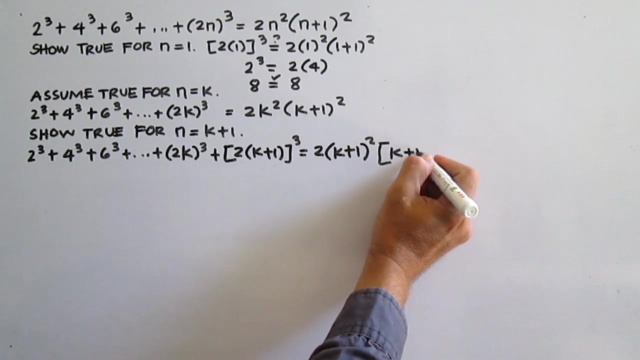 you, you, you, the next term, where n equals K plus 1 plus the cube of the product of 2, and the quantity K plus 1 is equal to 2 times the square of K plus 1, times the square of the quantity K plus 1 plus 1. 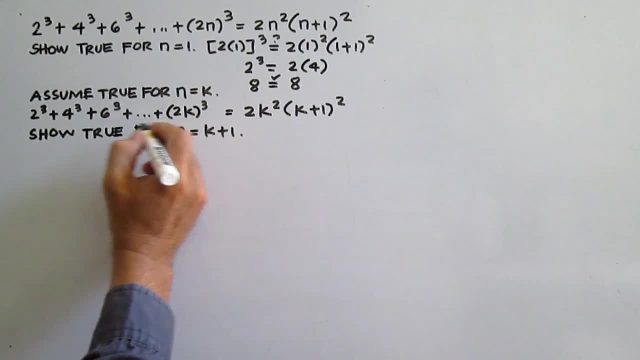 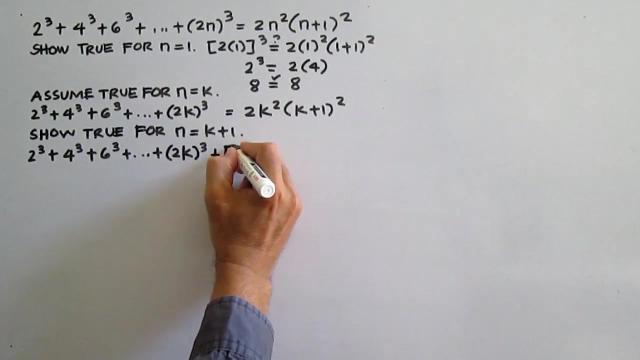 equals K plus 1. copy the left-hand side of the assumption. add the next term where n is equal to 2 and the next term where n is equal to 2. K plus 1 plus the cube of the product of 2 and the quantity K plus 1 is equal. 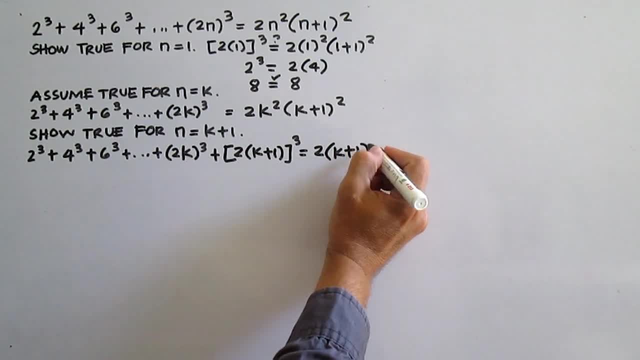 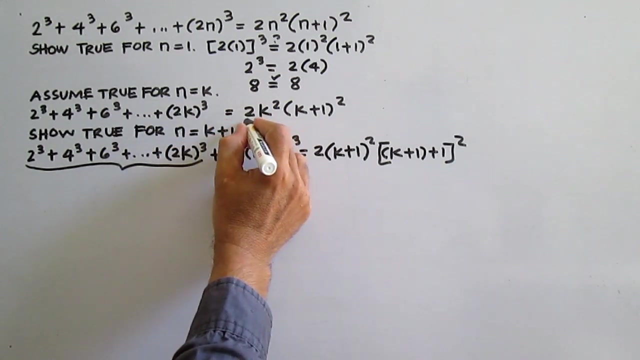 to 2 times the square of K plus 1 times times the square of the quantity K plus 1 plus 1. note that this expression is equal to the left-hand side of the equation in our assumption, which is equal to 2 K squared times the square of the quantity. 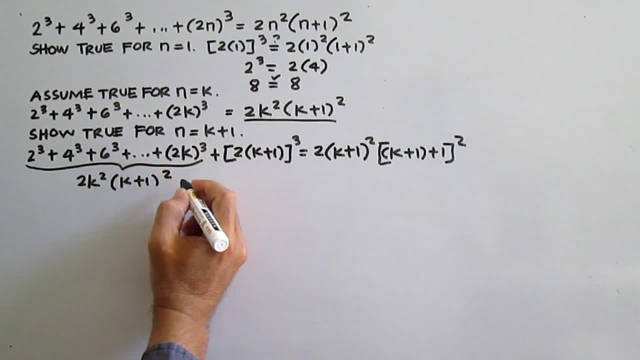 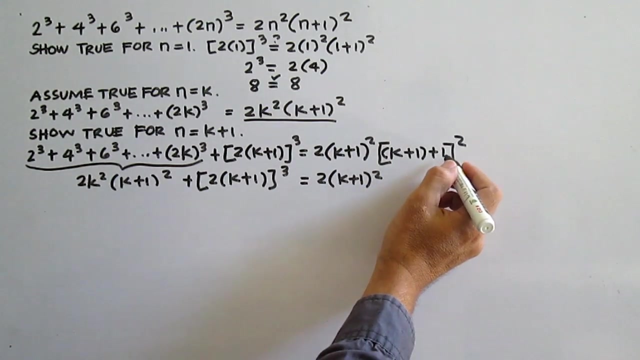 K plus 1 plus the cube of the product of 2, and the quantity K plus 1 is equal to 2 times the square of the quantity K plus 1 times the square of K plus 2. let us show that the left-hand side of the equation is equal to the right-hand. 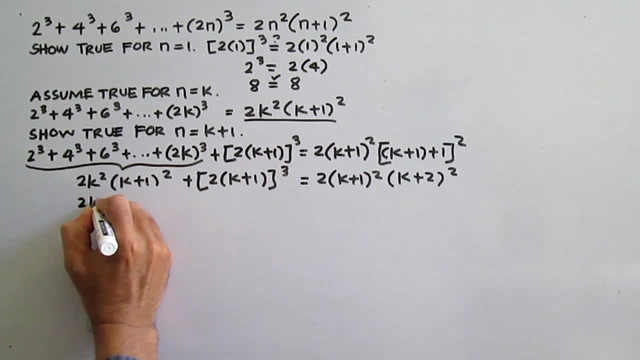 side of the equation is 2 K squared times the square of the quantity K plus 1, plus 2 cubed times the cube of the quantity K plus 1 is equal to 2 times the square of the quantity K plus 1 times the square. 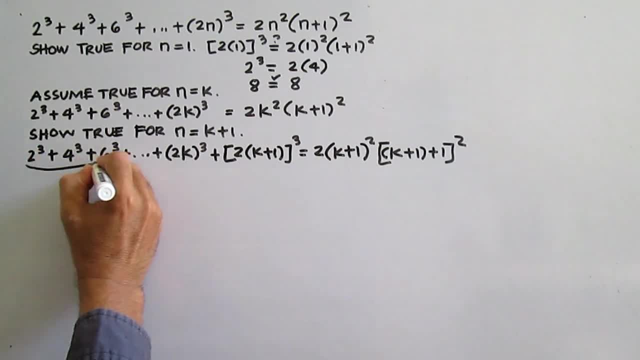 you Note that this expression is equal to the left hand side of the equation in our assumption, which is equal to 2k squared times the square of the quantity k plus 1 plus the cube of the product of 2 and the quantity k plus 1. 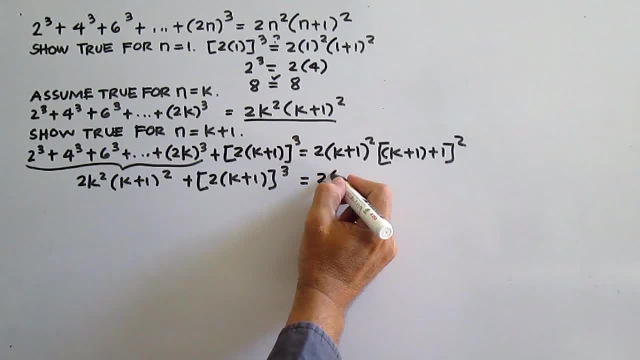 is equal to 2 times the square of the quantity k plus 1 times the square of k plus 2. Let us show that the left hand side of the equation is equal to the right hand side of the equation is 2k squared times the square of the quantity k plus 1. 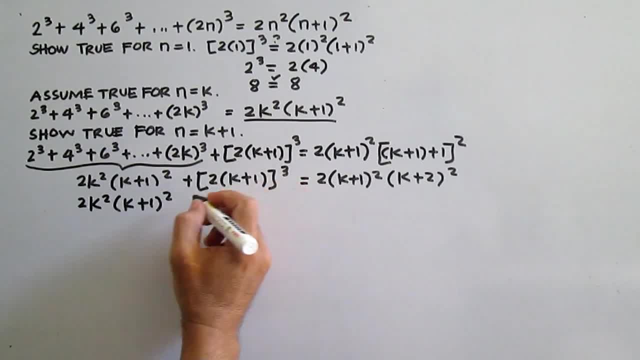 plus 2 cubed times. the cube of the quantity k plus 1 is equal to equal to two times the square of the quantity K plus one times the square of the quantity K plus two. factor out the square of K plus one and two. two times the square of the quantity K plus one, and the other factor is K. 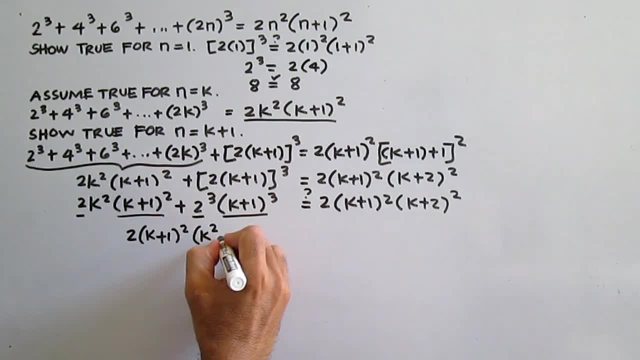 squared plus two squared times the quantity K plus one is equal to two times the square of the quantity K plus one times the square of the quantity K plus two. let's simplify: K squared plus two squared times the quantity K plus one, two times the square of the quantity K plus one. 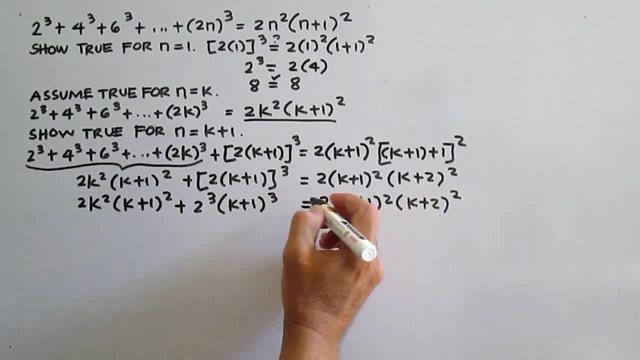 of the quantity K plus 2. you factor out the square of K plus 1 and 2, 2 times the square of the quantity K plus 1, and the other factor is Y. k squared plus 2, squared times the quantity k plus 1 is equal to 2 times the square of the. 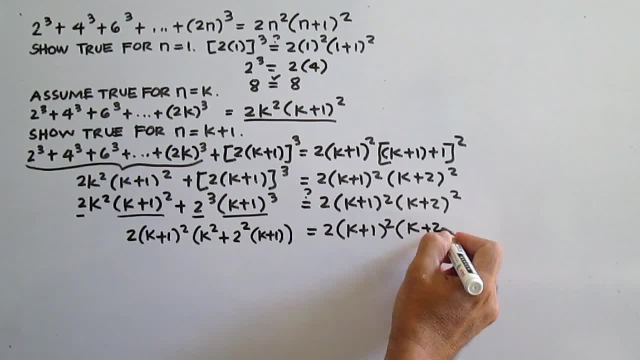 quantity k plus 1 times the square of the quantity k plus 2. let's simplify: k squared plus 2 squared times the quantity k plus 1, 2 times the square of the quantity k plus 1. times k squared plus 4k plus 4 is equal to 2 times the square of the quantity k plus 1 times the square of the. 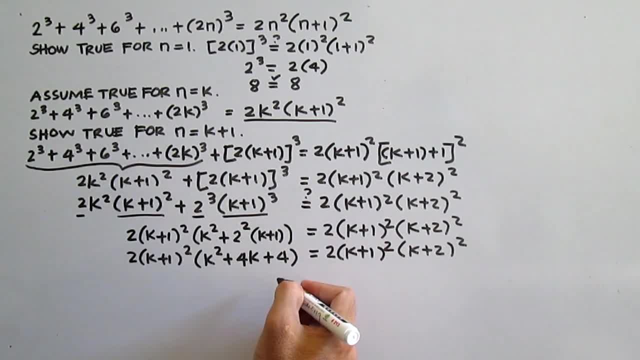 quantity k plus 2. a squared plus 4. k plus 4 is a perfect square trinomial which is equal to the square of k plus 2, 2 times the square of k plus 1 times the square of k plus 2 is equal to 2 times the square of the quantity k plus 1 times the square of the quantity k plus 2. 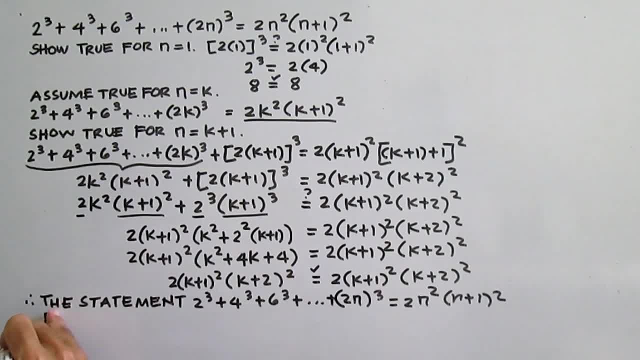 true, or the statement: 2 cubed plus 4 cubed plus 6 cubed plus dot dot dot plus the cube of 2 n is equal to 2 n squared times the square of n plus 1. is true for all natural numbers N. thanks for watching.